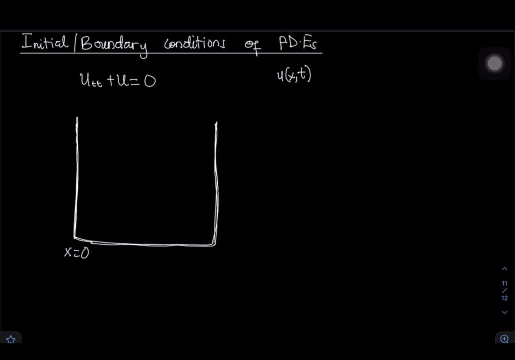 at x being equal to zero. that's one border, and i can also have the behavior of the solution. when x is equal to l, okay, and the solution, or the behavior of this solution, you know zero, maybe t is going to be equal to a function of t and then u of l, t that's going to 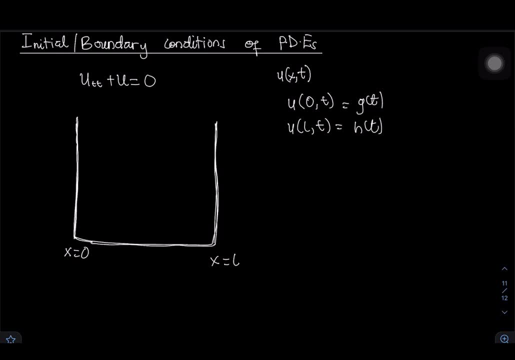 be a function of t. okay, these are known to be the boundary conditions. these are boundary conditions, so the boundary conditions actually tell you the behavior of the solution at the borders of the. you know the domain. now, this part of the domain is also going to be: when time is equal zero, what's? 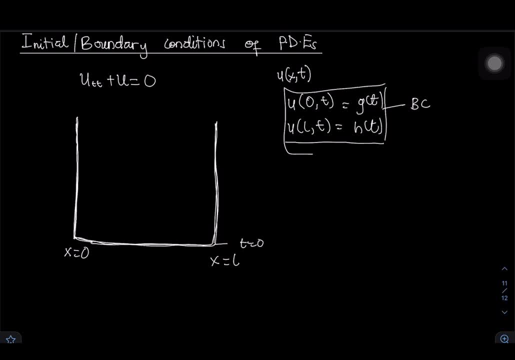 the solution like that's: t equals zero. what's the solution like? so, for example, let's say we, we are talking of diffusion, okay, and at time, equals zero. let's say there was, let's, let's, let's pick, you know um. let's say a glass of water, okay, and then let's say a bucket of water where you 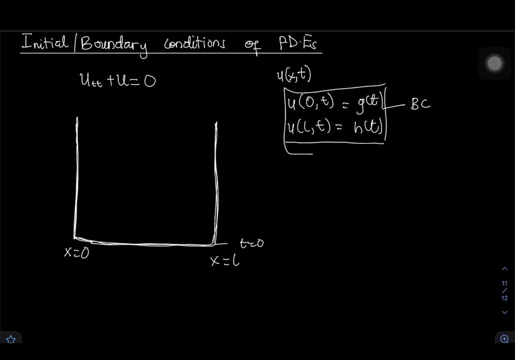 drop a solid potassium, potassium pair manganese into you. just drop this one into the bucket. then at time, t equals zero. you can see that this, this, this, this, this, this, you know, potassium permanganate is just going to be concentrated at one point, like at one point. 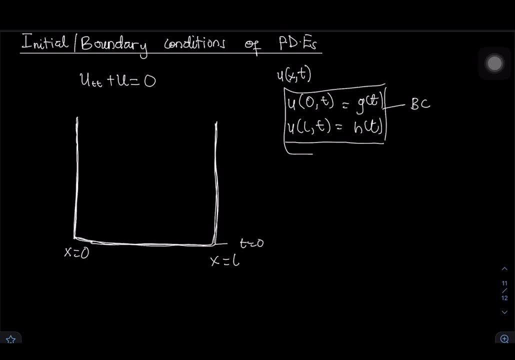 within the entire domain, right, and as time goes on, it's going to diffuse throughout the entire domain. okay, so at time t equals zero. what is the solution like? visually, you can see that the potassium permanganate is just concentrated at one point within the domain. and as time goes on, 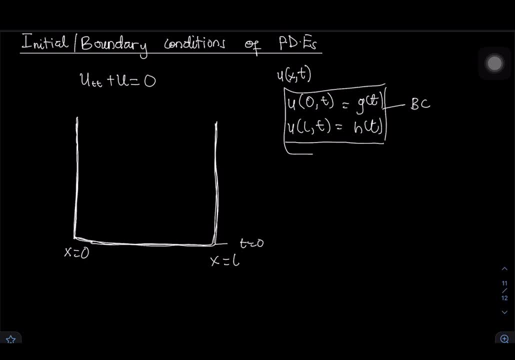 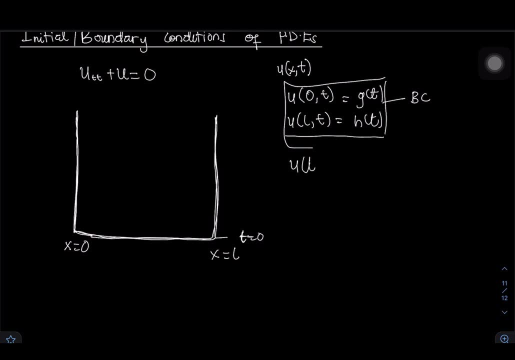 it keeps on to, you know, spread throughout the entire domain. so at time, t equals zero. what is happening? so at time, t equals zero. sorry, you can have some boundary. at some time t equals zero. let's say zero t, oh sorry. oh my god, sorry about that. u of x, zero. that's going to be some g of x. 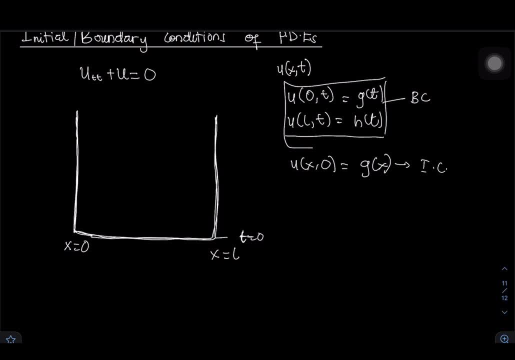 then this is an initial condition. okay, so an initial for initial conditions. you're trying to. you know you're trying to do something like this. you're trying to do something like this. you're going to check the solution, okay, at the beginning of time. so at time, t equals zero. what is happening? 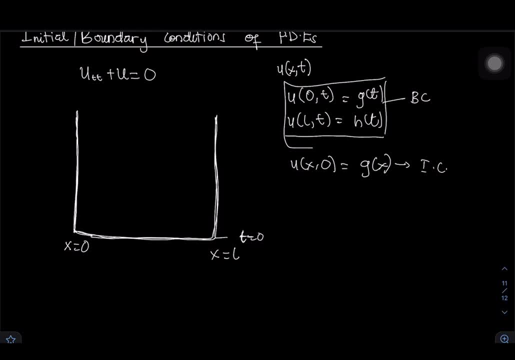 to the solution, that becomes a um, an initial condition. and when you are not fixing time, but then you go to the boundaries or the borders of this domain and check the solution or the behavior of the solution at these borders, then you're talking of boundary conditions. okay, yes, now these. 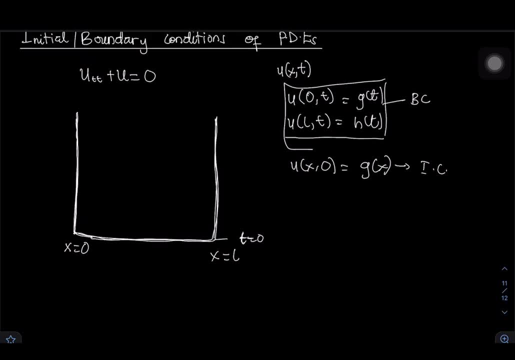 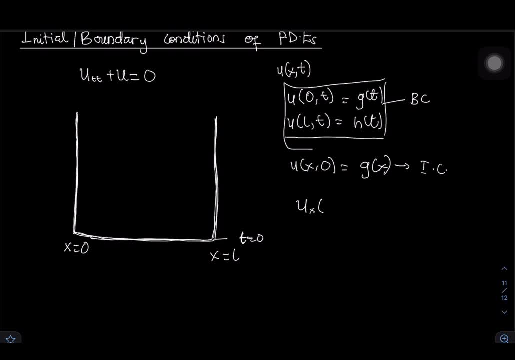 so is u x of. let's say no, let's say um. you know you. yeah, there's a u x of. you know x zero is equal to still g, maybe g prime of x. okay, this is still an initial condition, so we are not really um cornering ourselves to just the solution, but also its derivatives you can also find, you can also you. 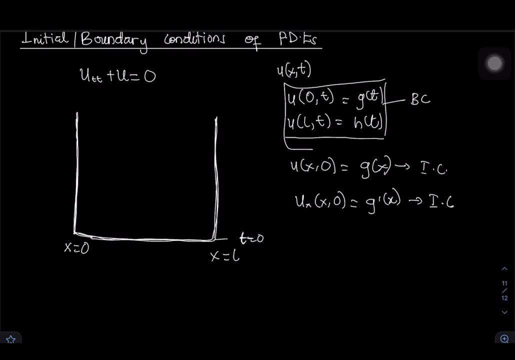 know, initialize the, the solution. that's even the derivative of, of of the solution at the beginning of time. it's it's kind of weird, but yeah that. so we are not just restricting ourselves to the u of x, zero, u of lt, no, we can also consider the derivatives of. you know the solutions at any. 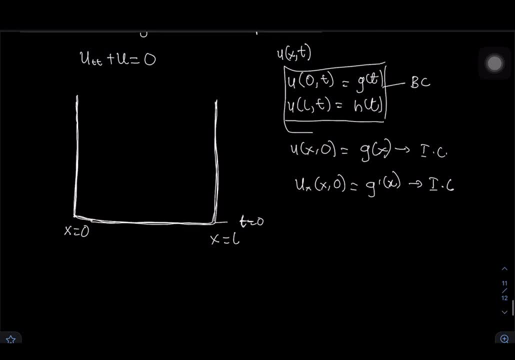 point in time. okay, so that's basically what boundary conditions are and what initial conditions are. um, initial conditions are just there, are no, you know um, um, how do i even put this? initial conditions are not really broken into other you know types. okay, an initial condition is just an initial condition, but for boundary conditions. 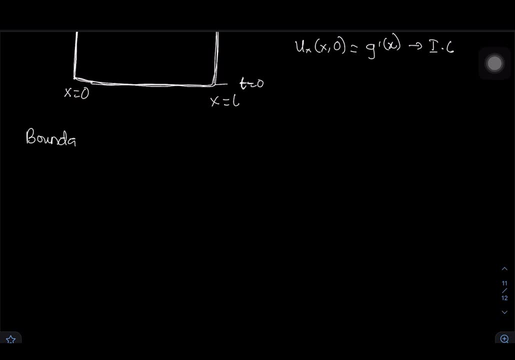 there are cases of boundary conditions and we are going to talk about them in this video. so the first type of boundary condition is just going to be the dirichlet, the dirichlet boundary condition. okay, so for the declare boundary condition, um, all we know is that, for you're just going to use. 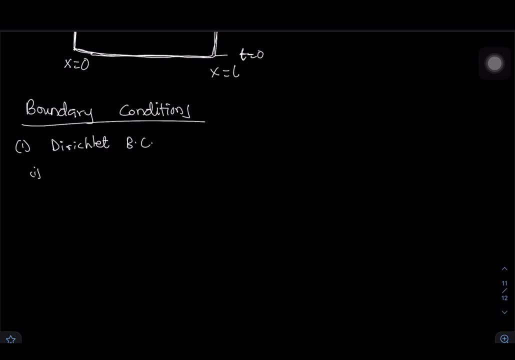 examples to make this one, these ones, you know, um clear. if i have the behavior of the solution, just a solution or the derivative of it, but the solution um at you know a point in space, g of t, then, or maybe the u of you know zero, t being equal to some h of t, or let me call it, maybe l, yeah. 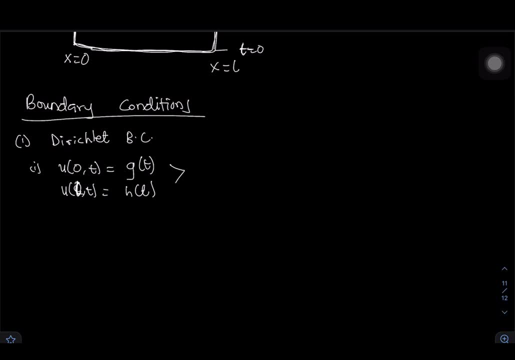 i used l right, so this one is l h of t. then these are called the dirichlet boundary conditions. you don't have any derivative of the solution at a point in space, but then it is just the solutions at the borders of the um of the domain. then that is a dirichlet boundary condition. 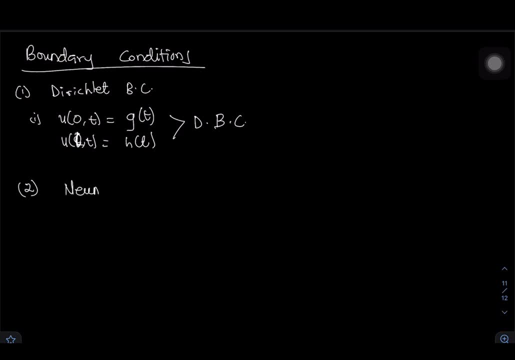 now number two. we are going to talk of the neumann boundary condition, and here you have the derivative of the solution, that's, the borders in space. okay, so example is just going to be ux of zero, t being equal to maybe a capital g of t, u x of l t, that's going to be capital h of t, and that we call. 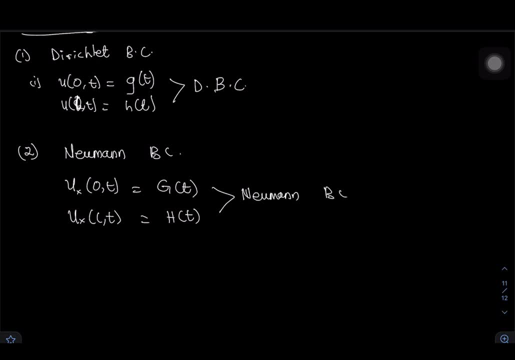 the neumann boundary condition, okay. and then now we have the robin. okay, let me not talk about it robin first. let me talk about the periodic boundary conditions. so with the periodic boundary conditions, what happens at border is happening at the at the other border. so here i'm gonna have 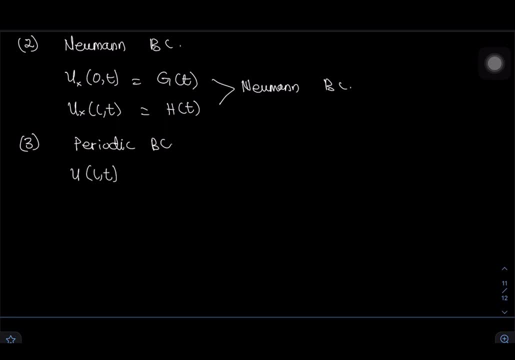 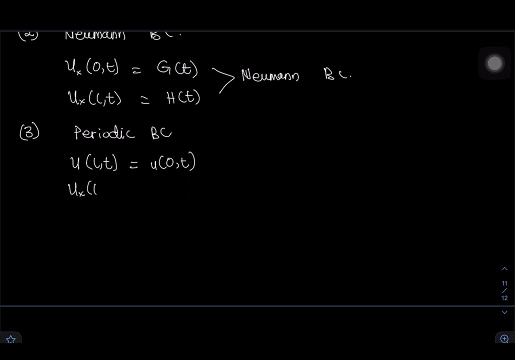 u of l t, which is the solution, or the behavior of the solution, at the border, one of the borders, which is the l. when x is equal to l, and that should be equal to u of zero t, i can also consider the derivatives of that: u, t, u x, of l t being equal to u x. 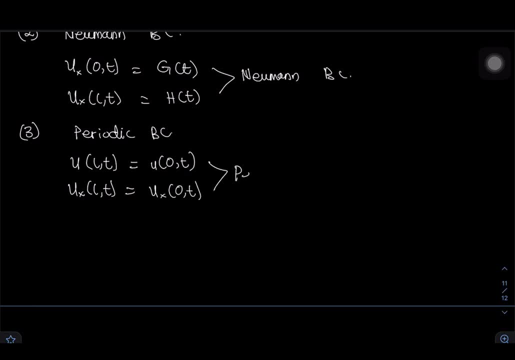 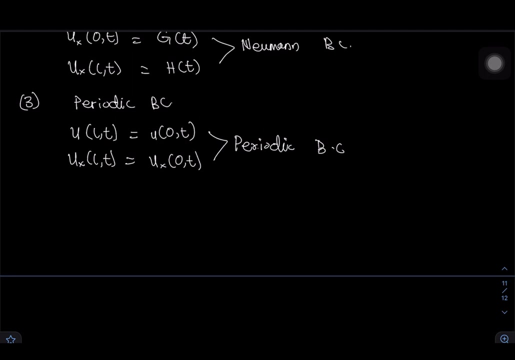 zero t. so this is going to be the or this, what we refer to as the periodic boundary conditions. what happens at one border or at one boundary, the same thing is happening at the other, and it includes the derivatives as well, and for the robin boundary conditions, which is a bit tricky- 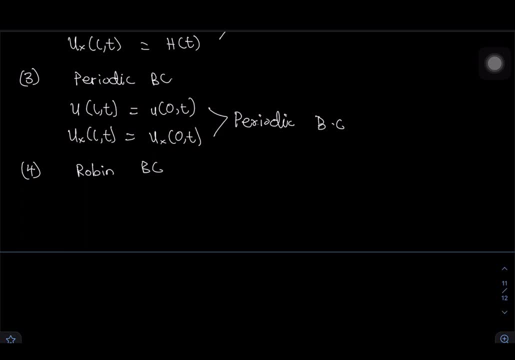 but uh, um, you're gonna have mixed derivatives over here. okay, you're gonna have mixed derivatives. you're gonna have- or it's a mixture of um of the solution itself, and then the derivative of the solution at one point of the or at points or at the borders of this um domain. so i'm gonna 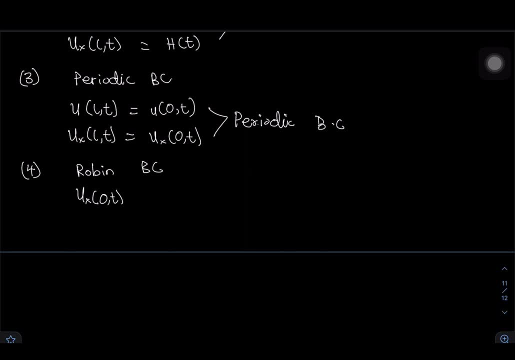 have u? x of zero t plus a? u zero t being equal to function of t, or you, oh my god, u x of you know l? t plus b? u zero t being equal to x of t. so here you can see that there's a mixture, there's a mixture of the derivatives, and then the solution itself adds some boundaries. 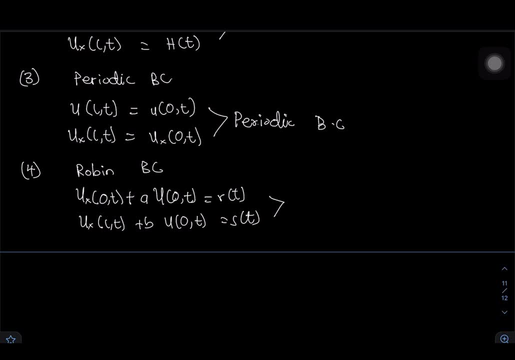 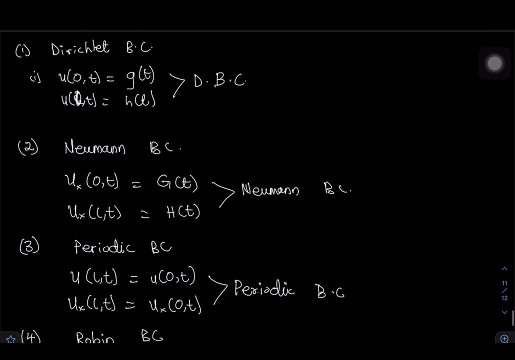 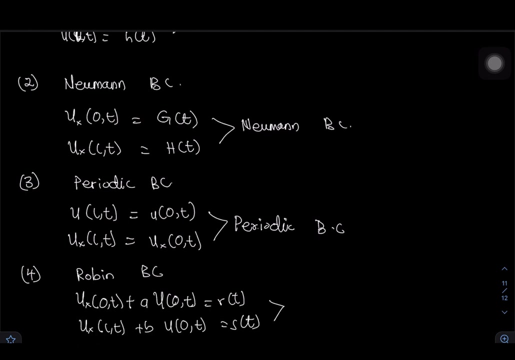 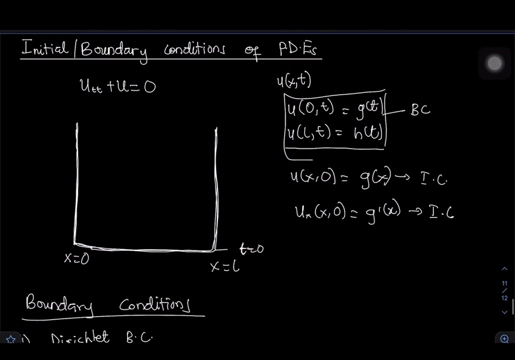 or some, some borders, and that gives you the robin boundary conditions. now, these are going to or. these boundary conditions are very crucial in our study of pdes, and then you'll see them in the later videos. okay, so, um, that's what i'm going to end with: the initial and then the 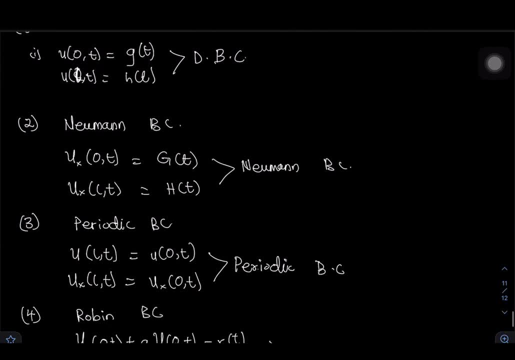 boundary conditions. now, in our next video, we are going to talk about well-posedness and um. i'd like to you to join me in that video, because that's all that. that's also one part, one interesting part about pdes and yeah, so see you in the in the next video and then, if you like the content.